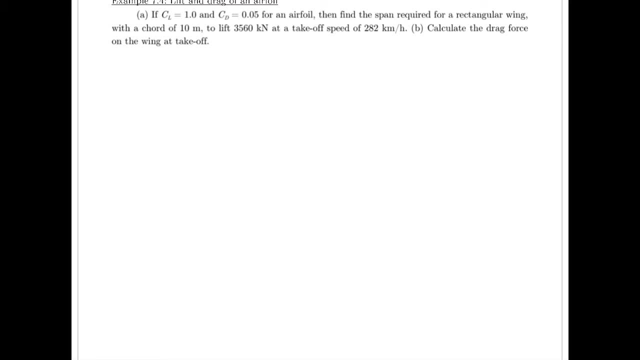 then find the span required for a rectangular wing. If it has a cord of 10 meters, it needs to lift 3,560 kilonewtons at a takeoff speed of 282 kilometers per hour, And then, part B, calculate the drag force on this wing at takeoff. Okay, awesome, That's a cool type of question too. 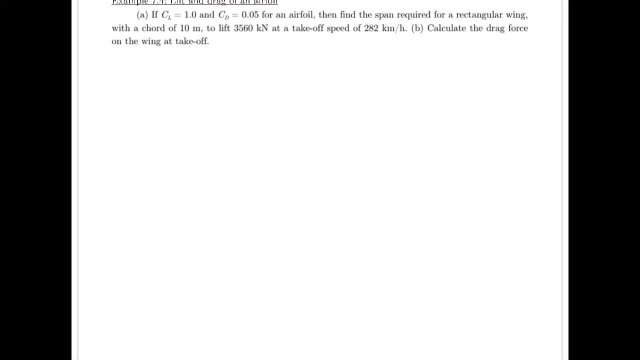 right. So it's saying: okay, for this type of airfoil we need this much lift at this speed. so how long does the wing need to be? You know? a nice practical application of this stuff, right there, right. So let's look at that. 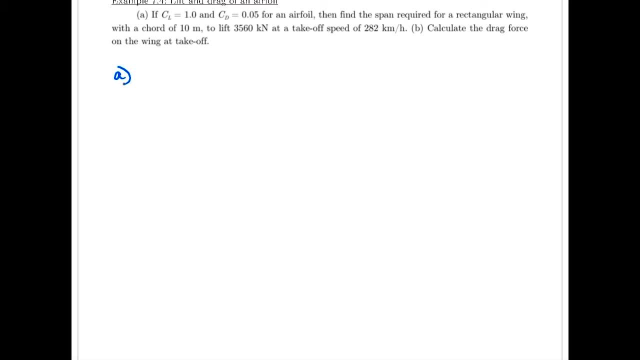 Let's look at A first. We'll remind ourselves of a few definitions maybe. So if we just sort of sketch out like a generic airfoil, like that, we remember the cord length was this distance, like across here. So that means, if we're looking down at a rectangular span, that might look like that. 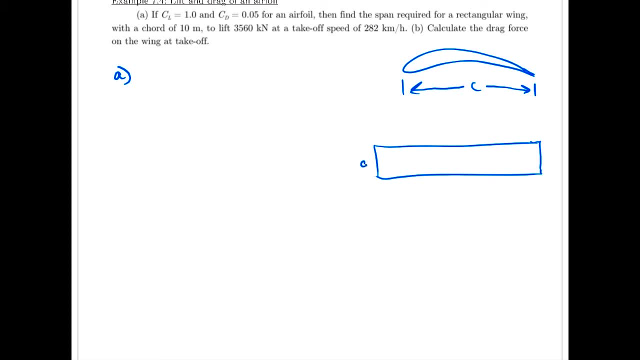 for example, right, that C from overhead now is going to be this distance here, that cord length, And we've called this B in our notes for wingspan right. So we'll look at the total wingspan there if we have a nice rectangular area And that is the. 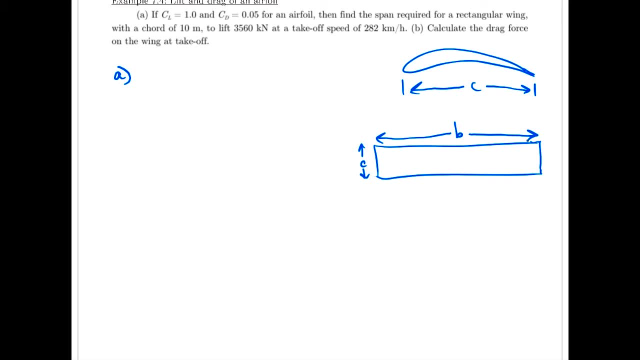 value we need to calculate. So first we write down our lift force expression, right, And that was just. lift force equals our lift coefficient, So the non-dimensional lift force half, and then it's rho V squared A. Sometimes you see that like a little P there for planform area. 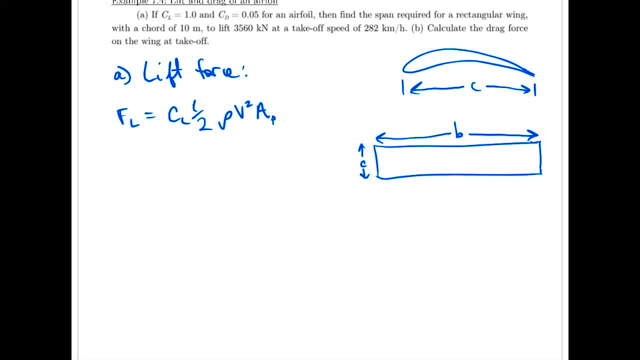 that's just this area we've sketched at the right here, Looking down on the wing, it's B times C right here. Okay, so now we just sub in right, So we can do like a quick conversion. You can do that. 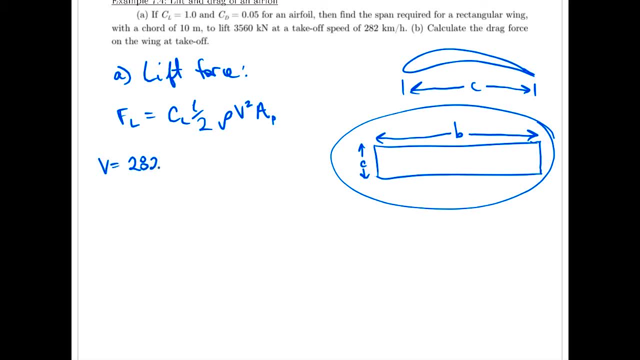 however you like. So V is 282 kilometers per hour, So you can do that conversion however you like. I'll maybe show you the long way here, just so we have it. I would first convert the kilometers unit. So we would say like: 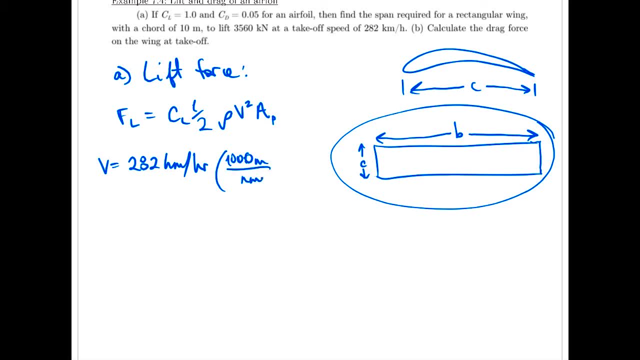 a thousand meters is going to cancel off the kilometers unit, And then I would do one hour on the top is 3600 seconds, 60 times 60, right? So then if you go ahead and plug all that in, you get 78.3 meters per second, which is the units we use it in, And you can see what I've done. 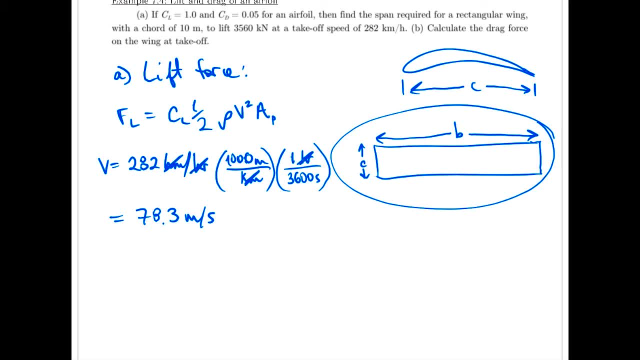 there. I've just canceled kilometers top and bottom and hours bottom and top, So you're left with units of meters per second, And you know what I mean. we usually have access to Google too. I mean, it pays to see how to do that, right, But in practice you can also quickly plug that. 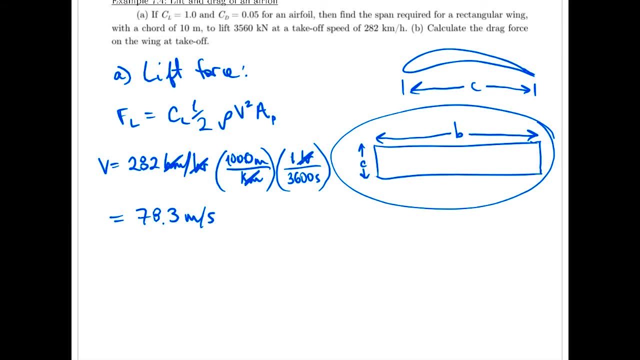 into Google, because that's what a lot of us do as well. That's a quick and easy way to do those conversions as well. So, marching through this, we have been given CL. We've got our V now, which was also given. We're going to need to calculate this area here, So density of air is the only remaining. 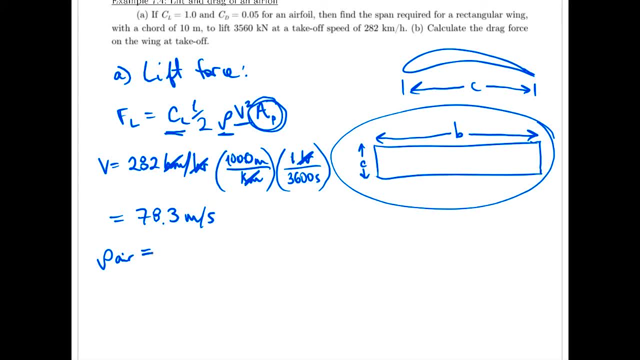 thing. So let's just list that out here. Density of air, Which, again, we can look up: 1.225, let's say, Kilograms per meters cubed. Okay. So lift force: we are also given right, We need to lift, that is our lift force. Speed given: We're even given. 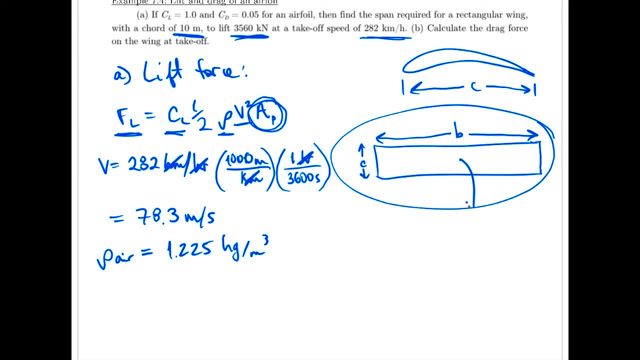 actually the cord right. So the planform area here, the area of the planform, is going to be B times C, where C is already given. So it's 10 meters times B, Alrighty. So we're going to sub in then for the lift force here and then rearrange, So CL half rho V squared B times C. 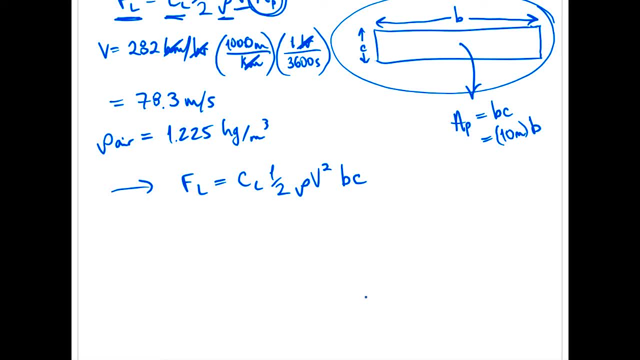 Scroll down here. Rearrange for B. B equals 2FL over CL rho C V squared. We sub in 2 times Okay, So that's the lift force here And then rearrange. So CL half rho V squared. B times C. 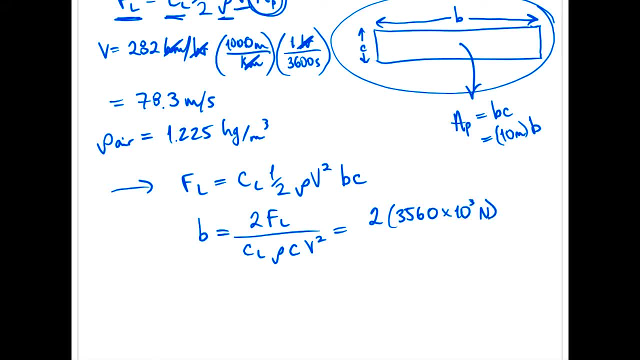 Scroll down here. We're even given. We're even given in kilonewtons, right. So let's get that to newtons so that we can balance our units. Lift coefficient given as well: 1.0.. Density, we've got. 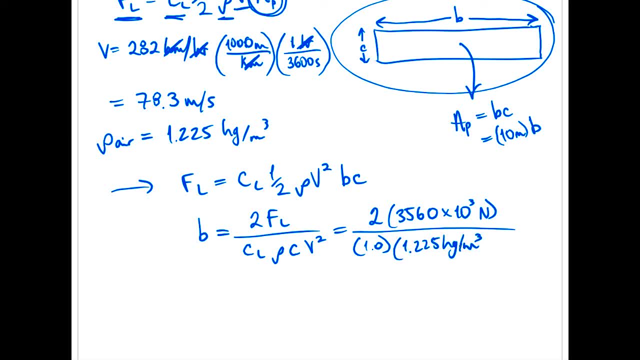 1.225 kilograms per meters cubed. C was given right 10 meters And V squared. what was that? 78.3 squared meters squared. Okay, A newton we remember is a kilogram meters per second squared. 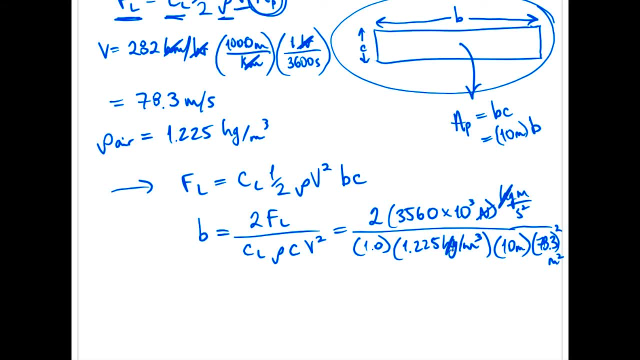 because it's a mass times acceleration. now we can cancel all these so that kilograms cancels. we've got a meters cubed on the bottom and a meters cubed canceling it out. oh yeah, my 78.3 was obviously meter squared per second squared. see that i would have caught a mistake there had. 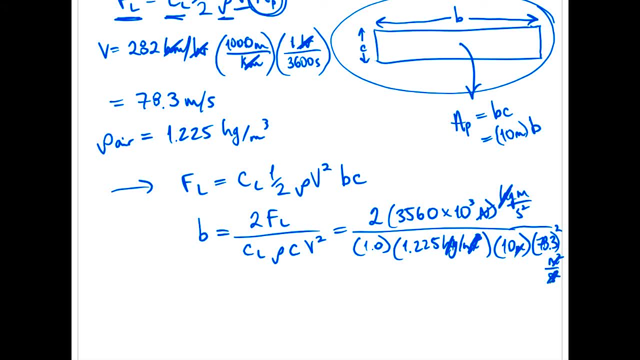 i made a mistake, turns out i just subbed in wrong for the units, so second squared cancels second squared, leaving us with meters, which is what we need. so it turns out the wingspan we need is 94.8 meters. okay, we box that off, of course, so everybody knows what our answer is. 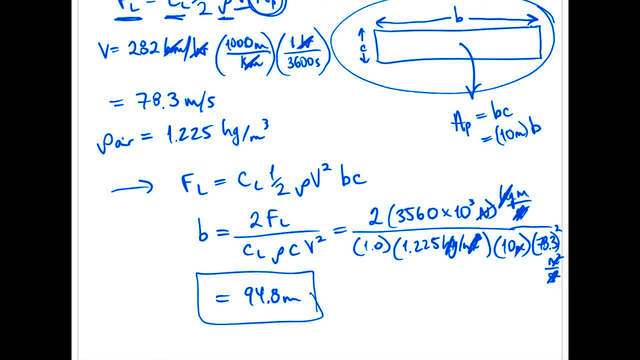 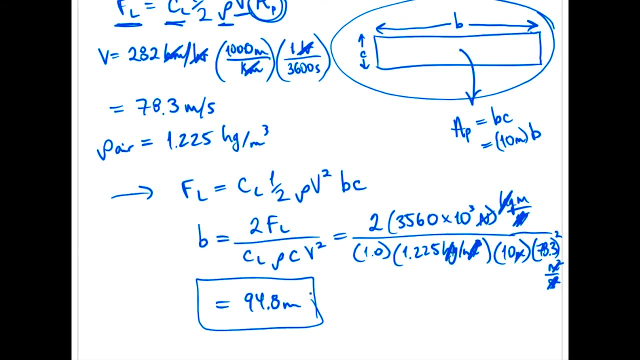 and ask ourselves if that makes sense. the cord is 10 meters long, so that's a big wing to begin with, so not overly surprising that we'd need you know 94.8 meters, uh, total length. that's a big aircraft and that's a lot of weight: 3560 kilonewtons. all right, so that's part a, part b, i'll just scroll up. 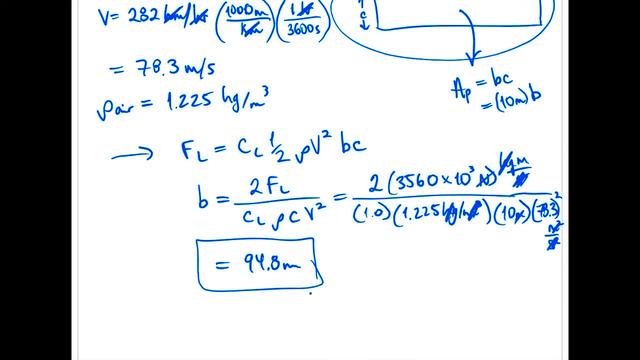 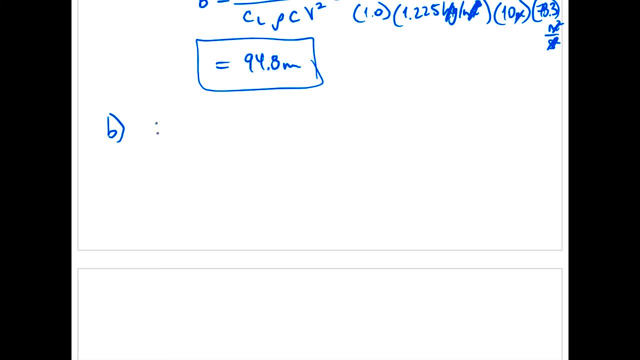 here calculate the drag force on the wing at takeoff. okay, so we go down. we're given our drag coefficient in this case, so that will be fairly straightforward, right? so we just write our expression. it's the cd half rho v squared a, so in this case that area is defined a little. 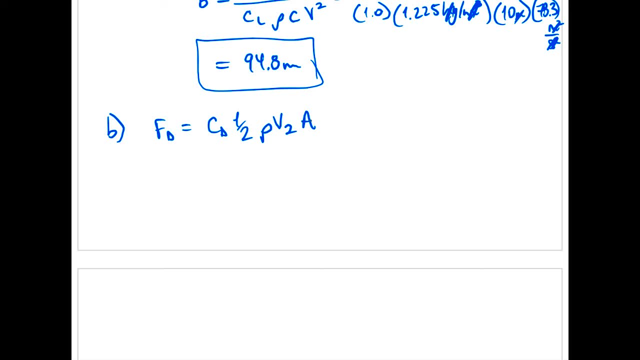 differently. we still use the planform area for the drag on the wing, based on the way this drag coefficient was given to us. so therefore, when we go into substitute- and, as i mentioned, this is generally dependent on where you get that drag coefficient from they'll- they'll tell you how it was calculated right, which area to use in. 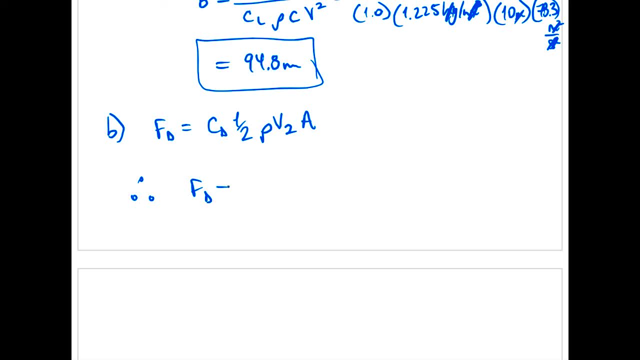 most cases. so don't worry yourself about that too much. so we can go ahead and plug in: 0, 0, 5 was our given drag coefficient. half density, again 1.225 kilograms per meters cubed. oh, i didn't write this correctly. let me fix that. it's v squared right, so 78.3 squared, and.